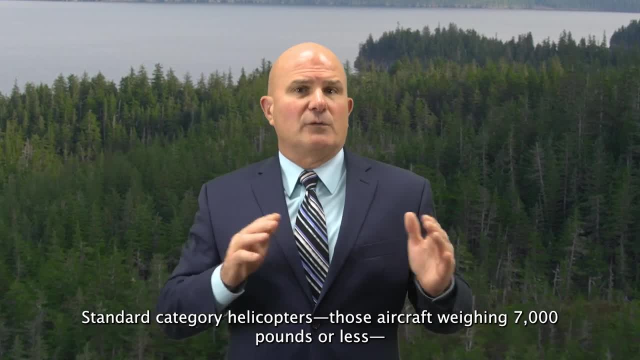 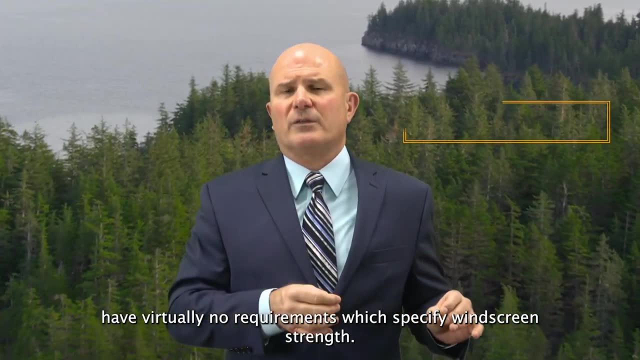 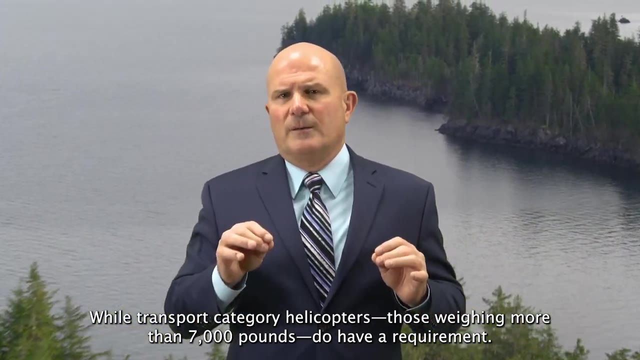 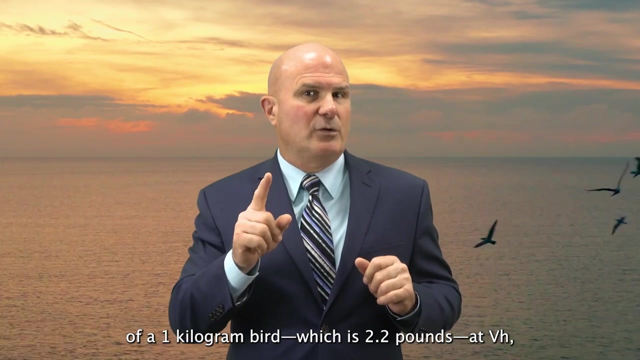 Standard category helicopters, those aircraft weighing 7,000 pounds or less, have virtually no requirements which specify windscreen strength, While transport category helicopters- those weighing more than 7,000 pounds- do have a requirement. Basically, the regulation states that the aircraft must be designed to withstand the impact of a one kilogram bird, which is 2.2 pounds at VH. 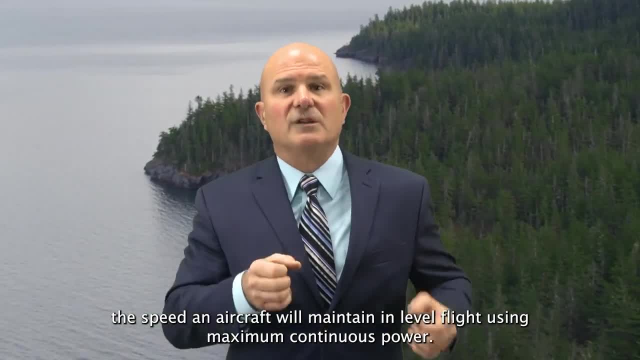 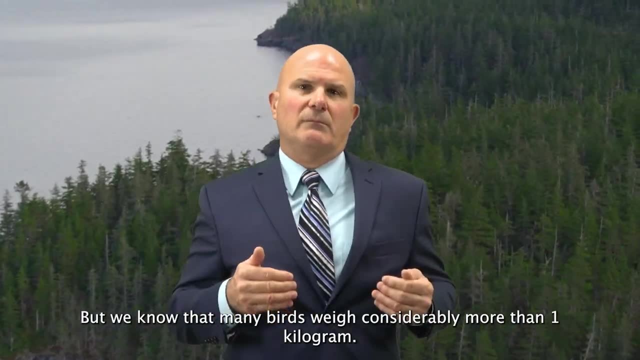 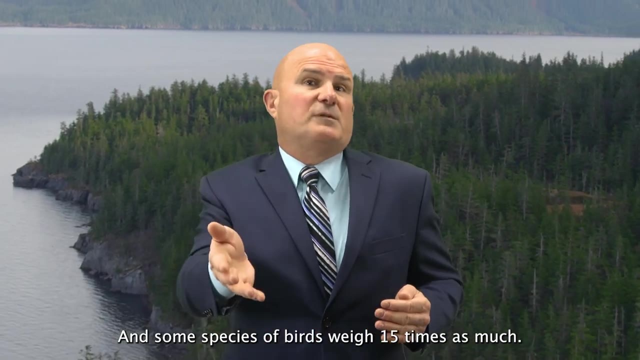 The speed an aircraft will maintain in level flight using maximum continuous power. But we know that many birds weigh considerably more than one kilogram. Hawks, eagles, buzzards, geese often weigh much more And some species of birds weigh 15 times as much. 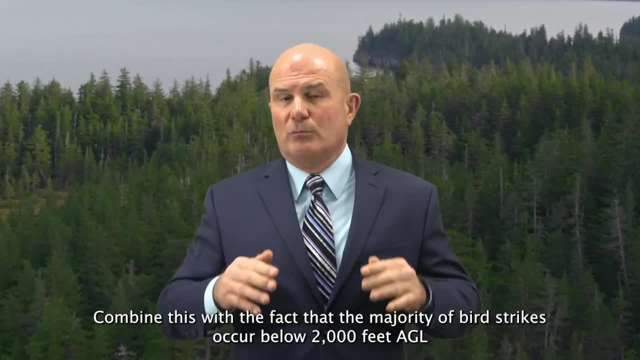 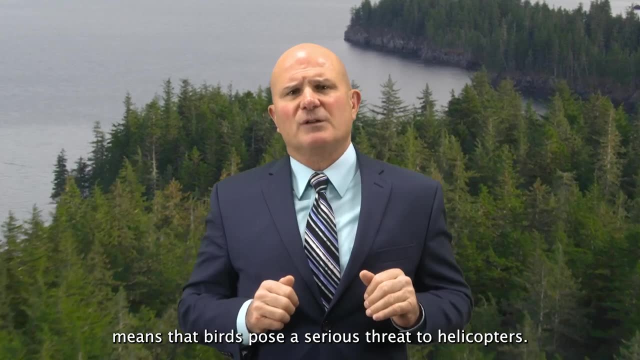 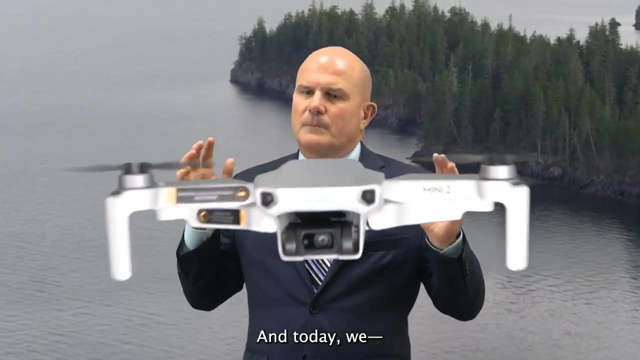 Combine this with the fact that the majority of bird strikes occur below 2,000 feet AGL in the same airspace we often use means that birds pose a serious threat to helicopters, And today we have the additional hazard of UASs Unmanned Aircraft Systems. 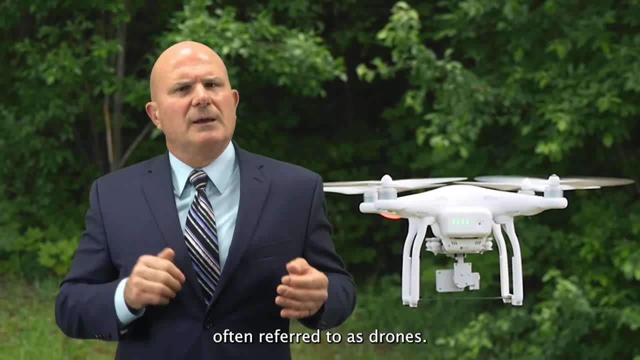 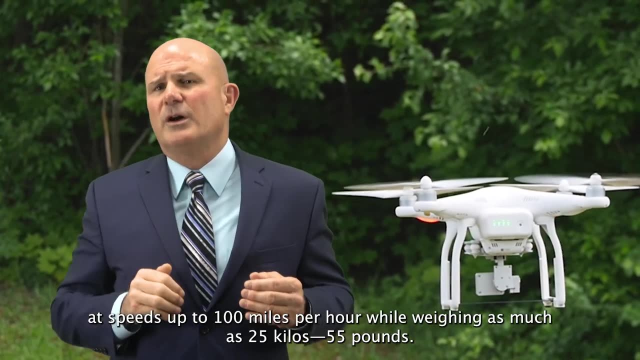 often referred to as drones. In most countries, these small drones are allowed to be flown as high as 400 feet AGL at speeds up to 100 miles per hour, while weighing as much as 25 kilos- 55 pounds. 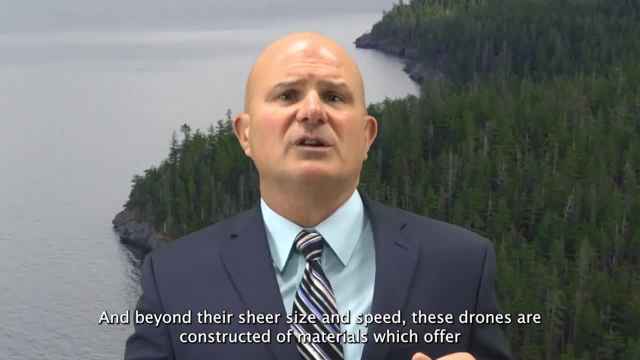 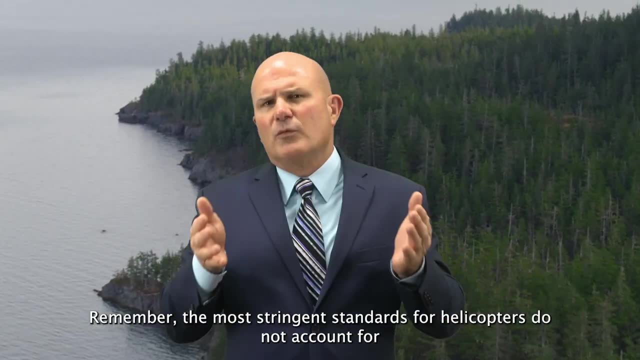 And beyond their sheer size and speed, these drones are constructed of materials which offer a much greater potential for aircraft damage than the flesh and bone of a bird. Remember: the most stringent standards for flying a drone, the most stringent standards for helicopters: do not account for a bird larger than one kilogram. 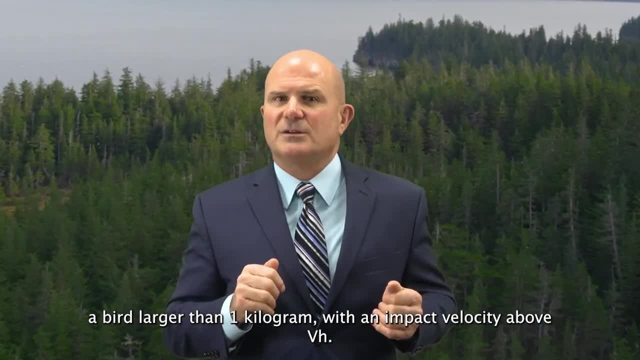 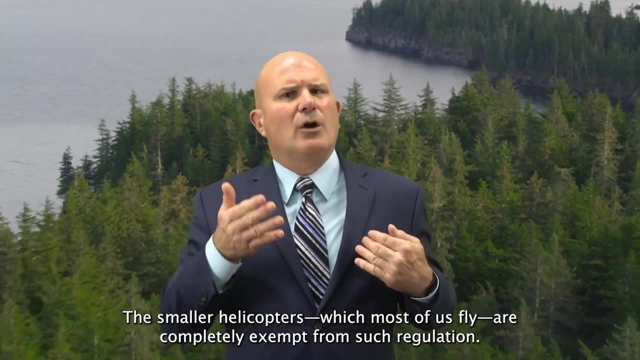 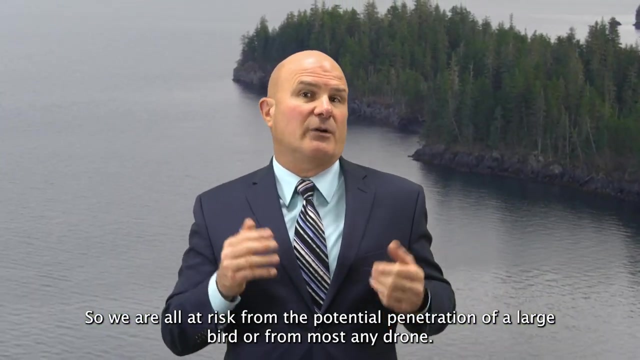 with an impact velocity above VH, And these are only required for transport category helicopters. The smaller helicopters which most of us fly are completely exempt from such regulation. So we are all at risk from the potential penetration of a large bird or from most any drone.